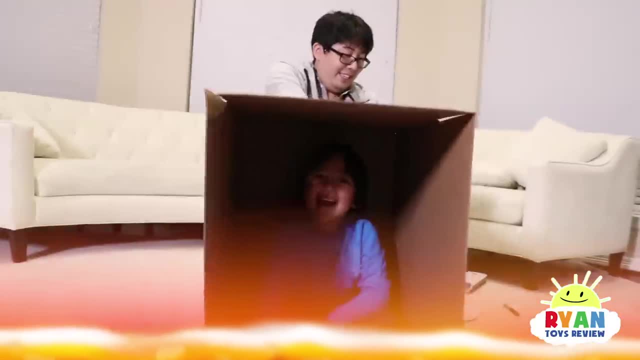 Secret base. Ryan hid somewhere and we have no idea where he went. Who's Ryan? Ryan make a noise. Where is he, I wonder He's in here? Nope, Nope, he's not in there, But it's closed off, so I don't know what to do. 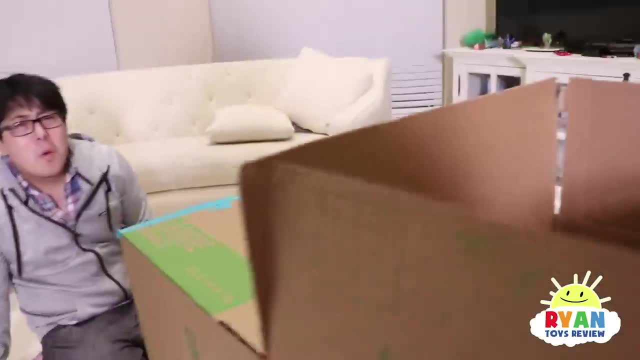 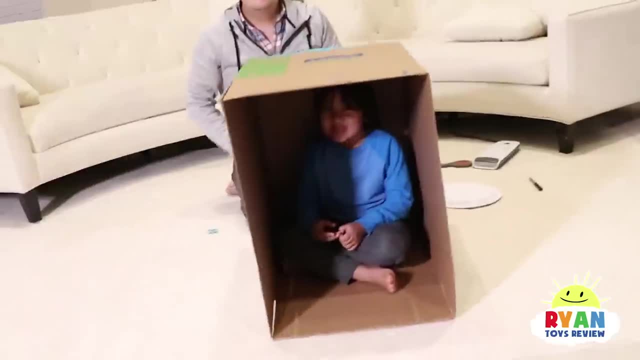 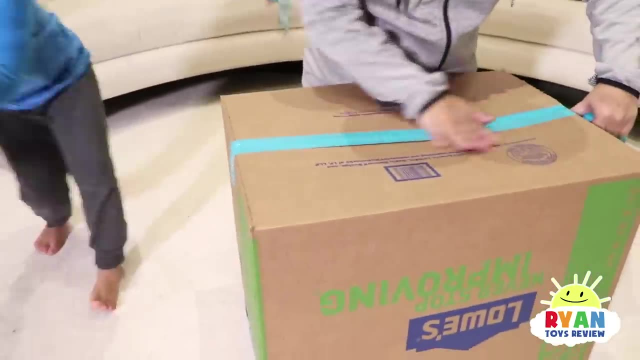 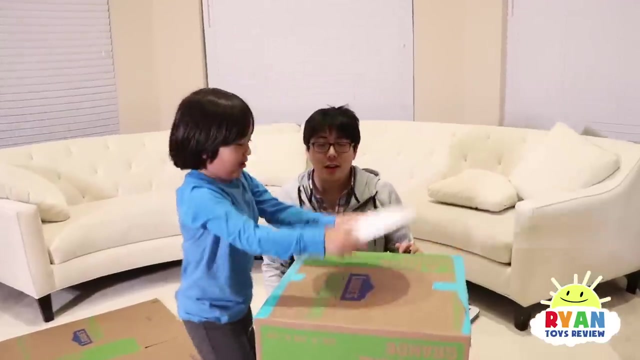 I think he's in this box here, Let's see. Let's see, Found you Taping the top side too, So I cannot get in. Yeah, No more getting in the box. Next we're going to make a hole in the box with this circle. 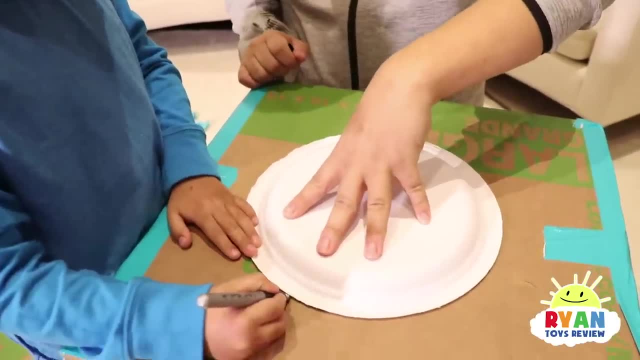 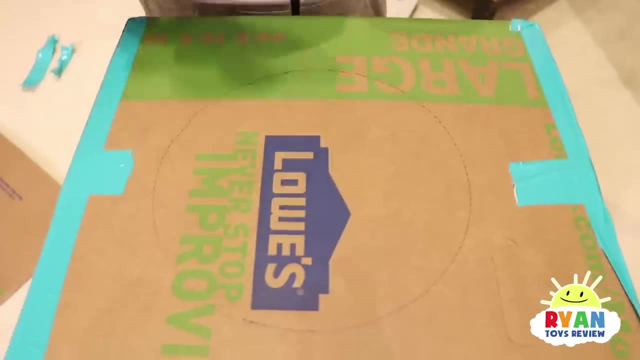 Alright, Ryan, Here's your pen. I'll hold the dish so you can draw the circle. Let's see Ta-da. Oh, Good, Good job, It's perfect. Oh, I feel like it's getting worse, Ryan. 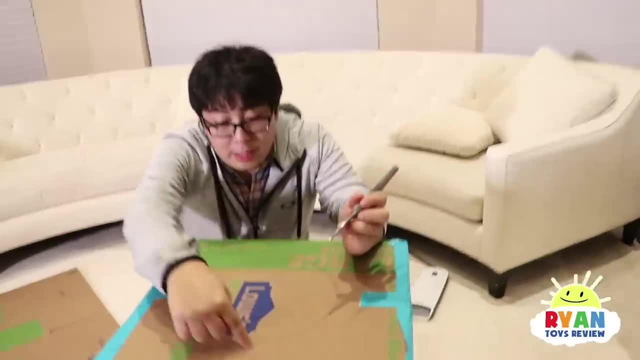 Now I'm going to cut it out. It's going to be very hard. Yeah, I'm going to cut it out of this circle. Dad's going to do dots first, then he has to make enough room for him to, Yeah, so this is probably a step for grown-ups, right? 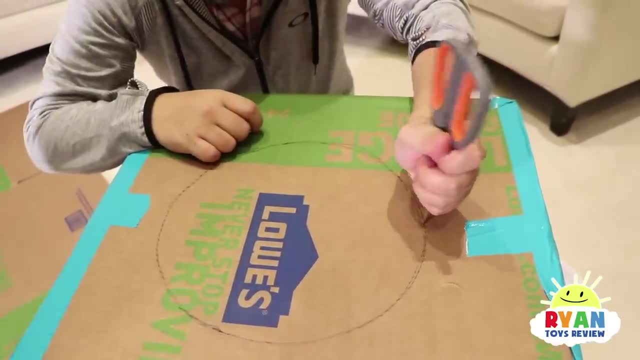 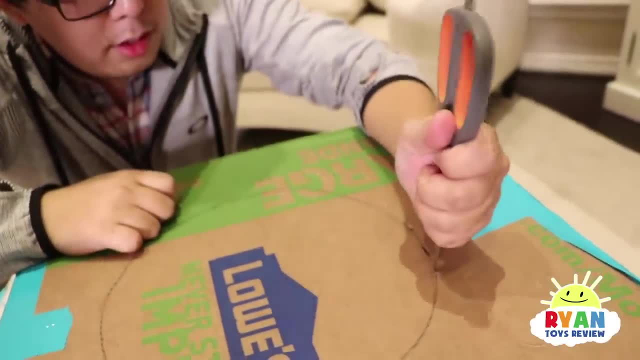 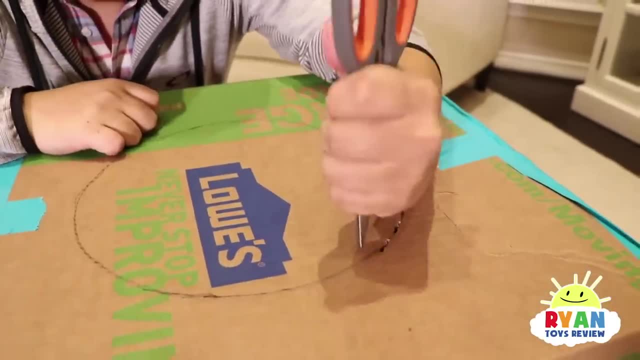 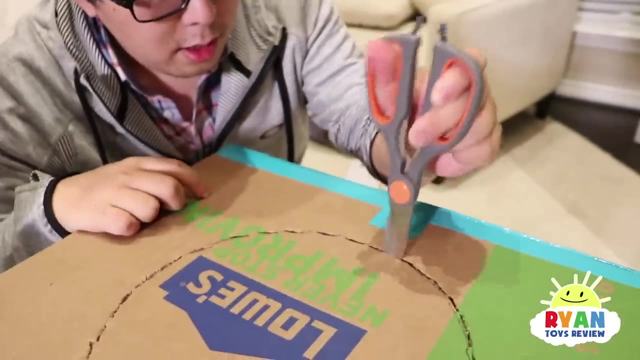 Even more time. Punch out the hole. Oh, Oh nice, Oh nice, nice, nice. Yay, Good circle, Good job. I think you're too big for the circle. Oh no, You fit. What if it shoots out you? 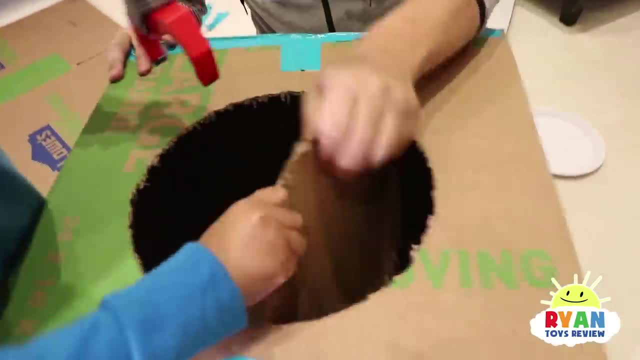 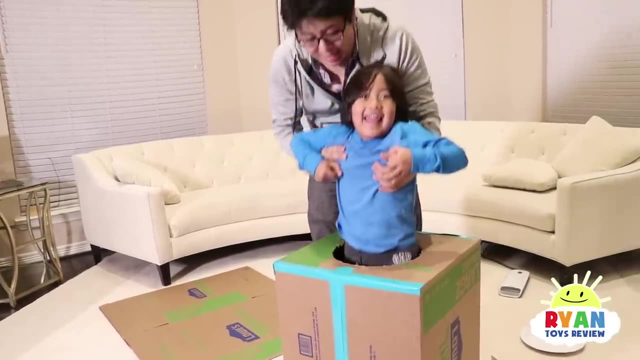 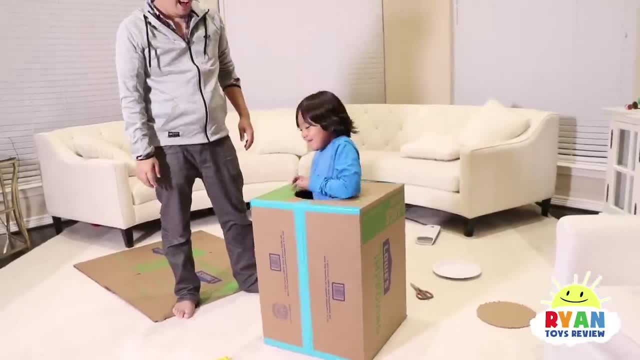 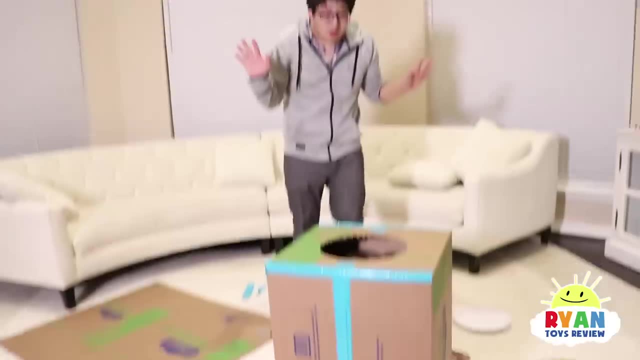 Oh no, Oh no, It shoots out. Oh no, It shoots you out. Oh no, Wow, Ha, ha, ha, ha ha. And this is an epic hiding spot. Oh yeah, Oh wait, where's Ryan? 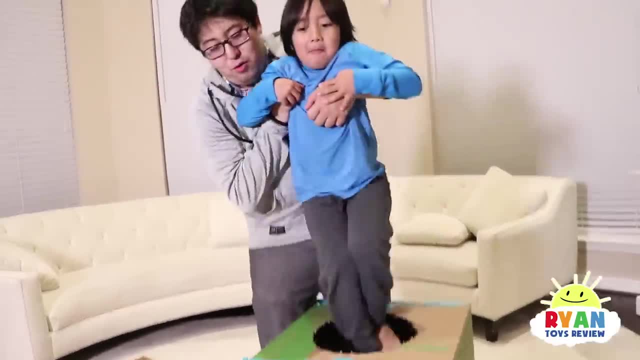 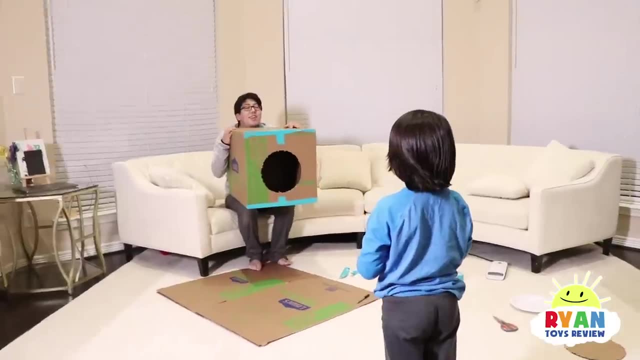 Where? Where's Ryan? Ryan, where, There he is. And then it shoots you out, po Whoo. Okay, kids, this is it actually. It's that simple. This is air bazooka. now You ready? Ryan. 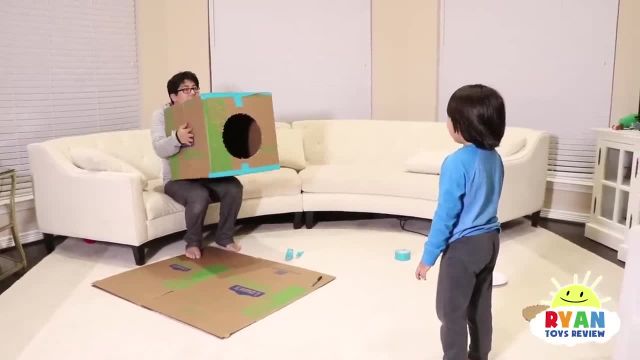 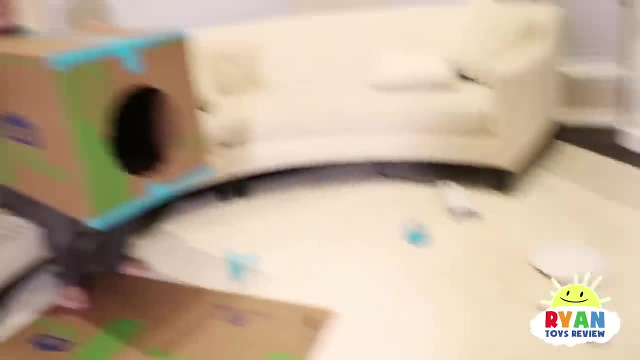 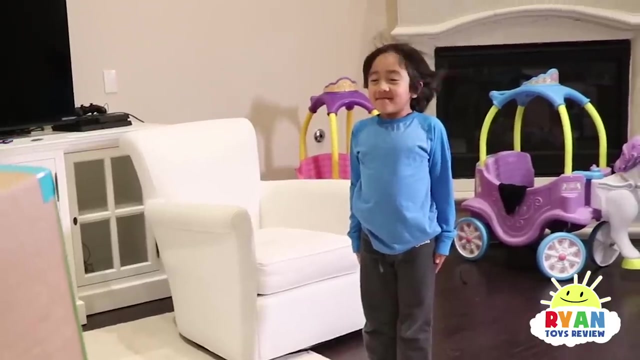 Yeah, Stand right here, Ready, two, one, Ah, Ha, ha, ha, ha, ha ha. That was actually air Really, Really, You ready? Yes, It feels good. huh, Wow, You feel the air. 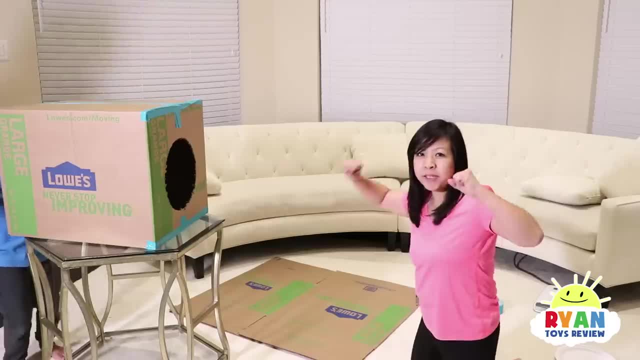 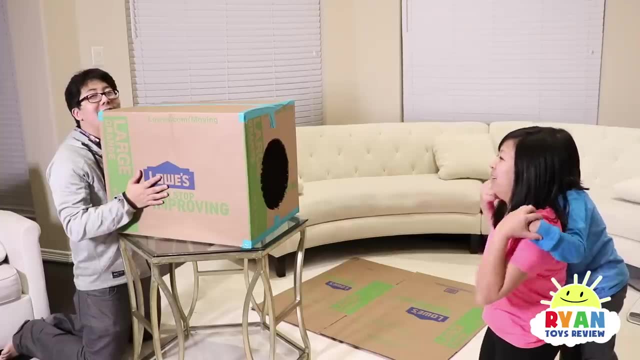 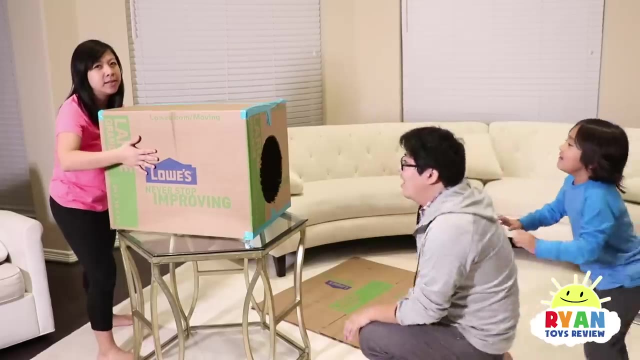 Yeah, try it to mommy. Okay, I wanna try, Mommy's gonna try. let's see if I can feel any air. Oh, a little bit Ready guys? No, All right, you guys, are you ready? 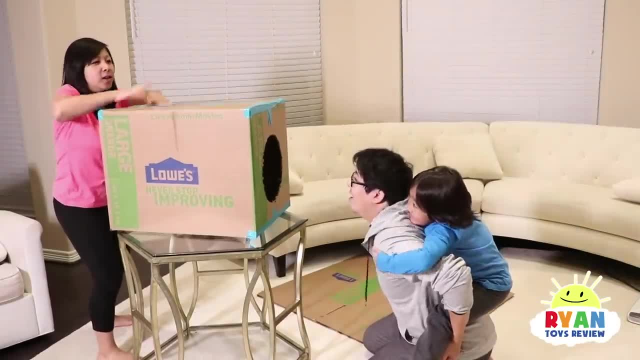 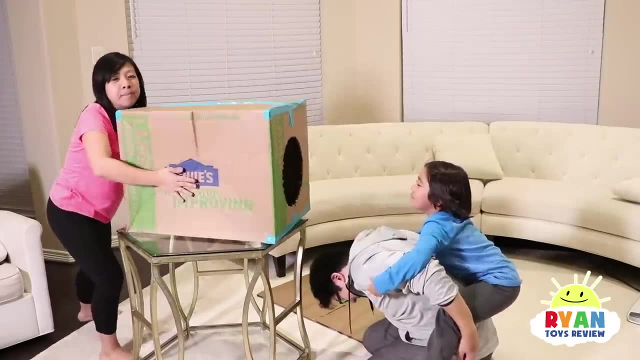 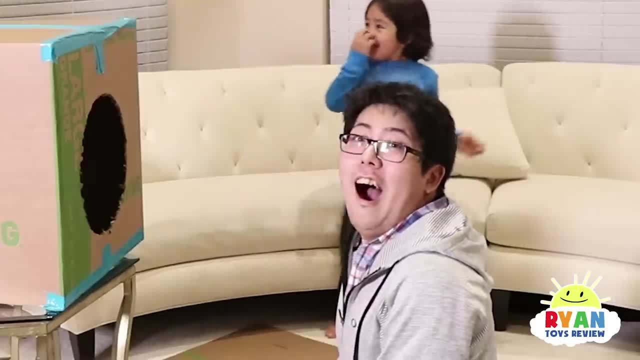 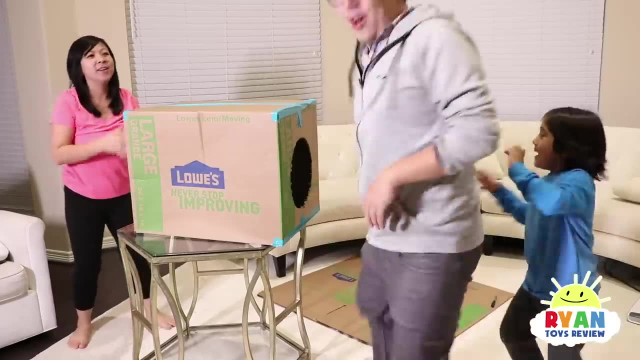 All right, here I need it. Oh, that was strong One in each other. Okay, okay, okay, have fun, My turn. Okay, Ah, All right, I got it. All right. let's see, don't run me. 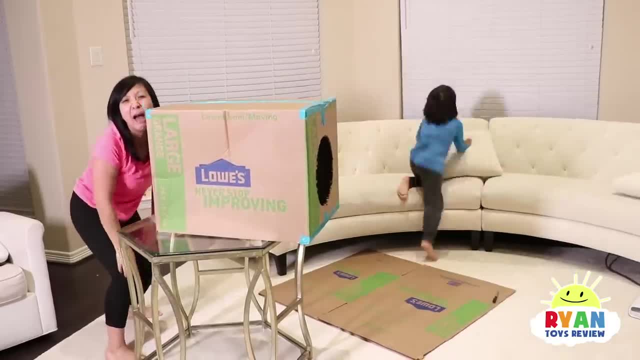 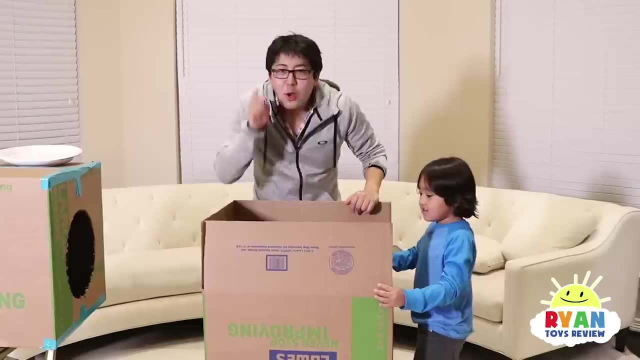 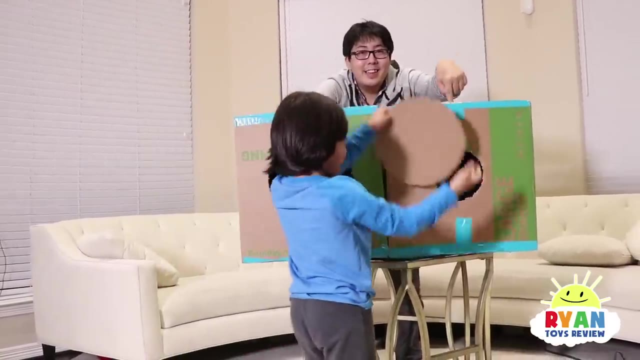 Ah Nothing, I'm not strong as daddy. that's why Now we're gonna make another bazooka, but with a smaller teeny hole, So we can experiment, see if it makes a difference. There's our two holes: a big hole and a small hole. 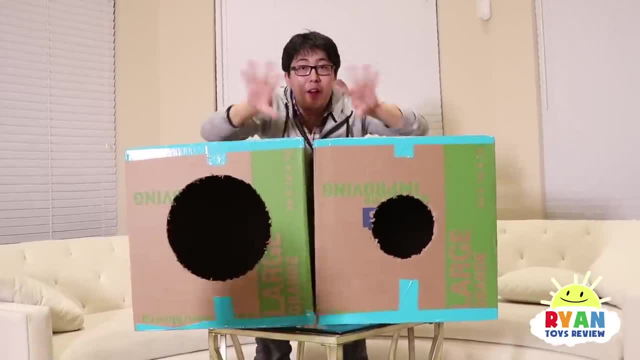 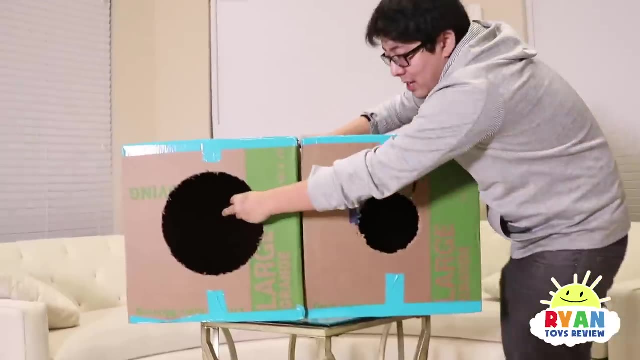 All right, and just to show you the difference between these two, how the air come out, I have this smoke machine here. I'm going to put smokes in these, But then we need to cover it, And then we cover it, and when we shoot, 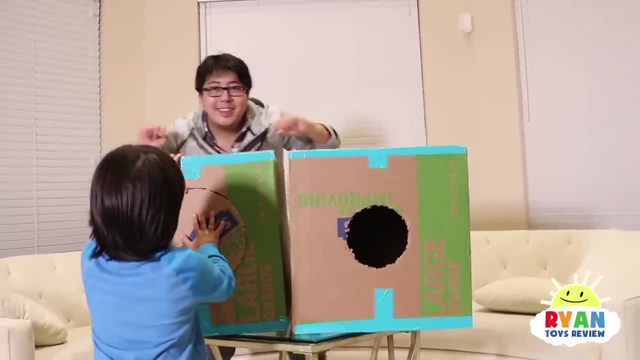 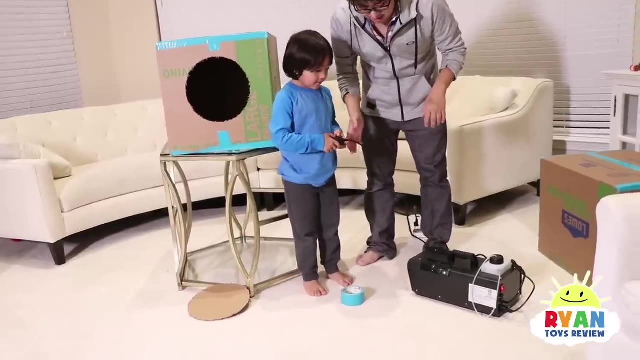 you can see the smoke come out and you can see how the air moves out of the box. Yeah, so it's called a vortex generator. Oh, that's cool Sounds, fancy, huh, Fancy. Turn it on, All right. 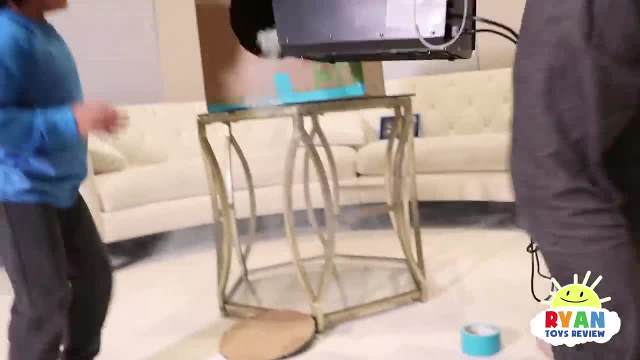 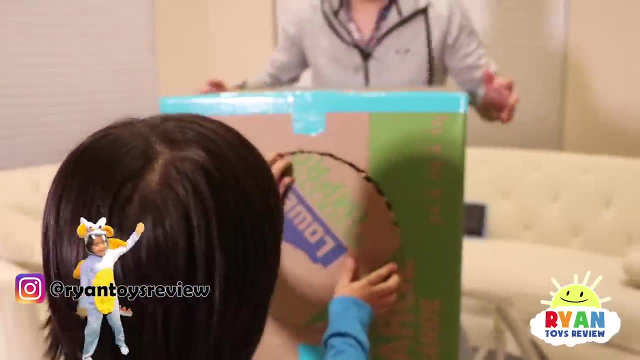 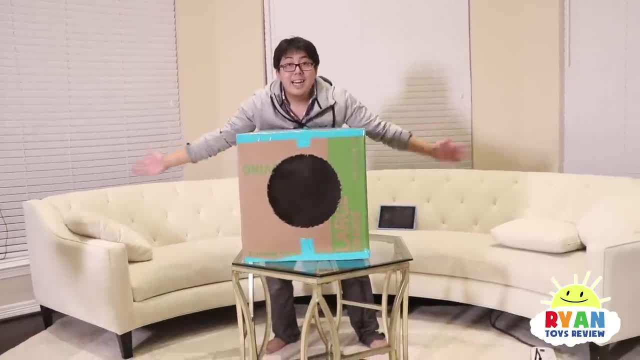 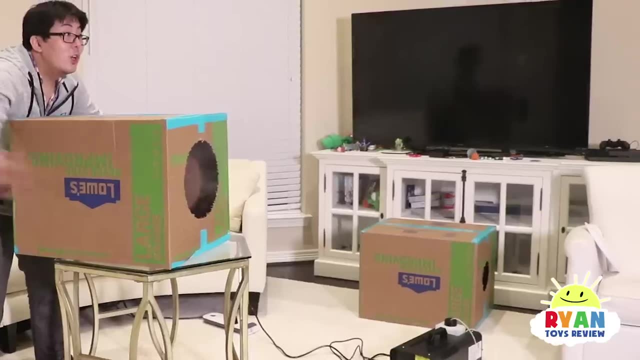 OK, I'm going to shoot at you camera. All right, let's see. Wow, What Did you see it? Yes, It looks like a fireball. It looks like a fireball. Wow, Wow, See, it looks like a fireball. 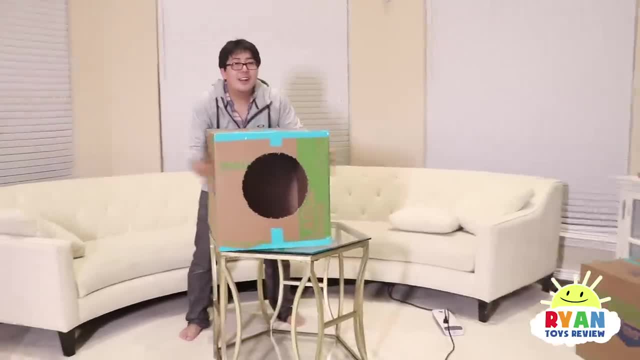 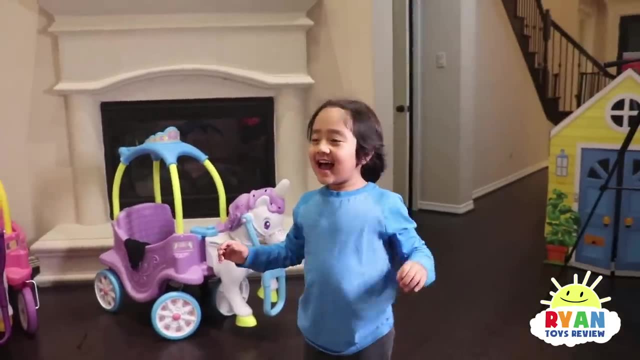 Whoa, whoa, whoa, Whoa. I want to try. Oh, I feel the air. Wow, Whoa, Do you feel the air? Now it's your hair. That was a big hole. Now we're going to try a small hole. 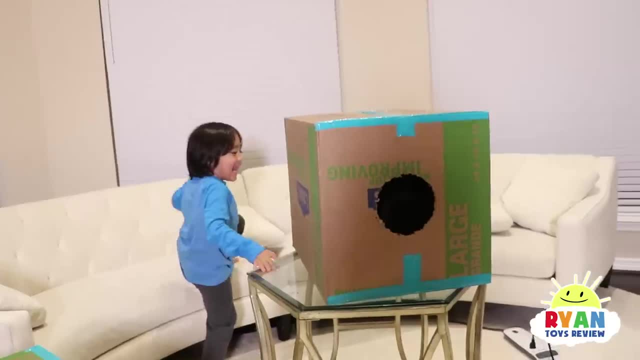 Yeah, let's see what the difference is, And I'm going to be first. OK, Oh, you want to try it? OK, Yeah, It's going to look very nice. Oh, this one. I can't even put the smoke machine inside. 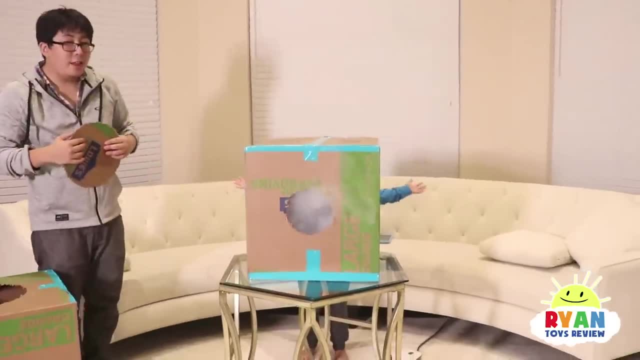 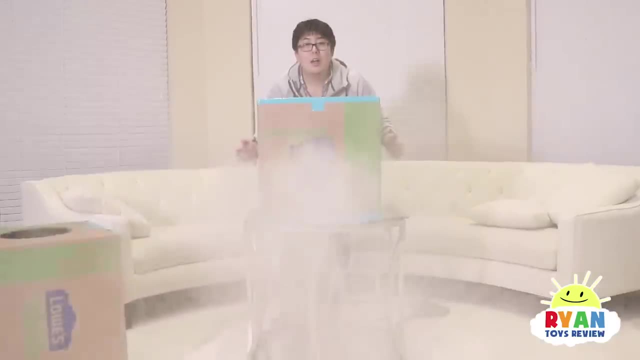 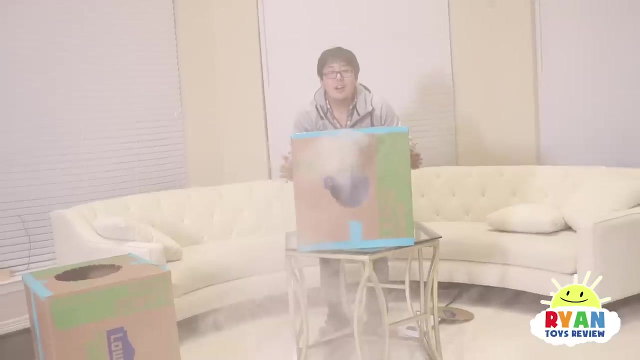 Oh, we're done. Check it out. OK, go ahead. Wow, You see it. Yes, Wow, this is stronger. It looks like a snowball. Wow, Dad, you look. Wow, I'll just slow it down. 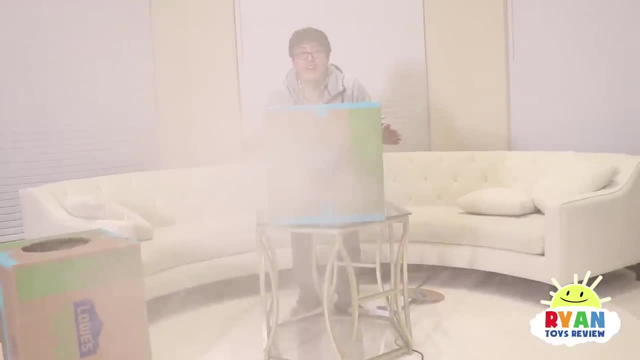 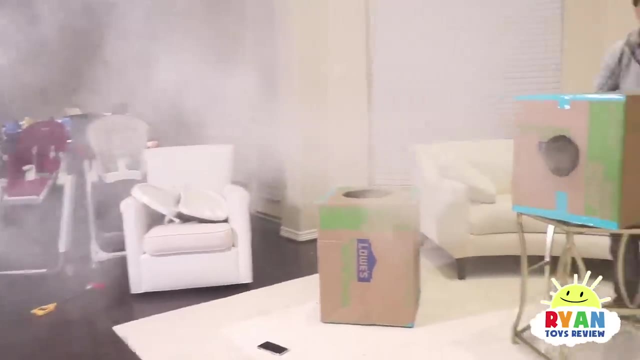 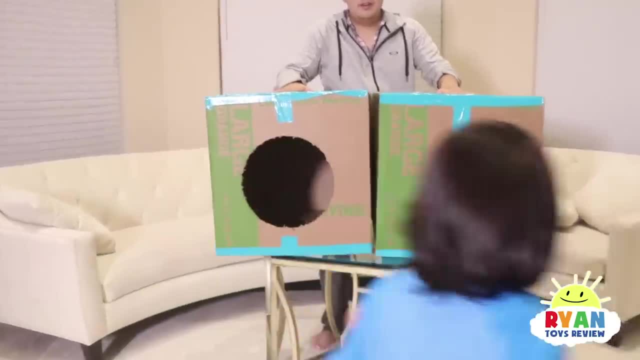 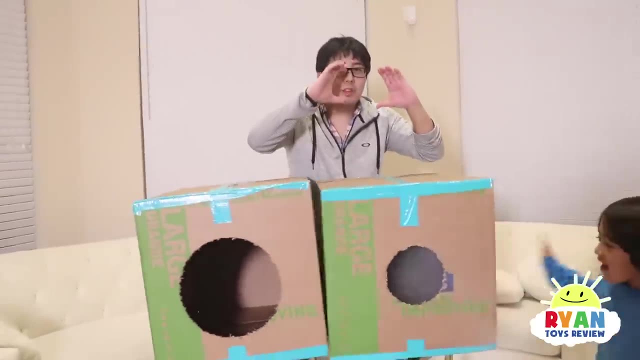 After this fun science experiment: which hole produces the stronger vortex? This one, Yeah, That's right, A smaller hole. It's smaller, so it's more concentrated. It still come out. huh, Yeah, There's still some in there. 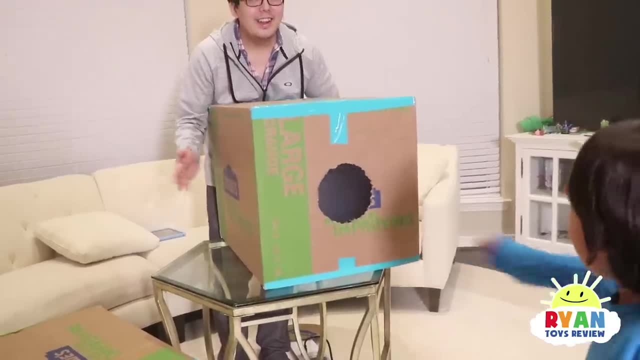 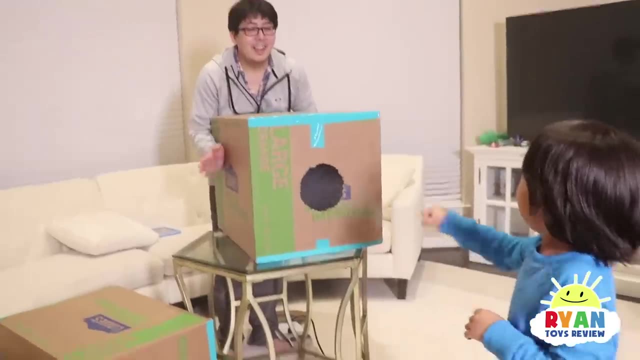 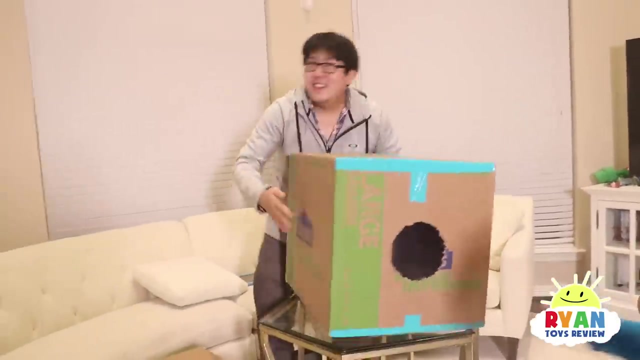 This experiment is best done outdoors because you don't want to trigger the alarm system, But we have ours turned off, so it's fine, You want to jam to it, Daddy? Now we're going to use air bazooka we made to see if we can put up the fire on the candle. 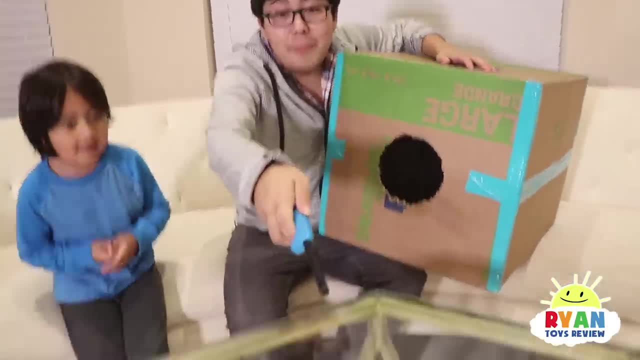 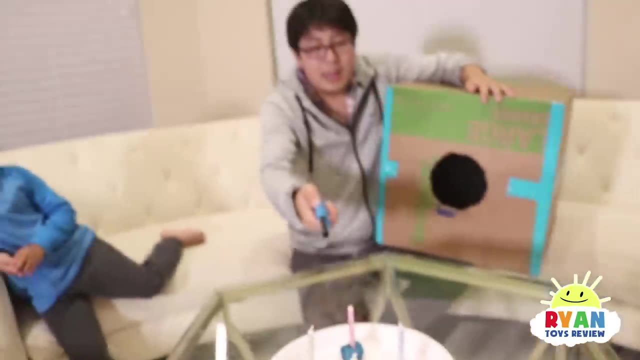 This is just birthday candles, right? This is just birthday candle that we used, and then we just used Play-Doh to make it stand. Let's light it up. Happy birthday to somebody. Happy birthday to nobody. Everybody, If today's your birthday, happy birthday. 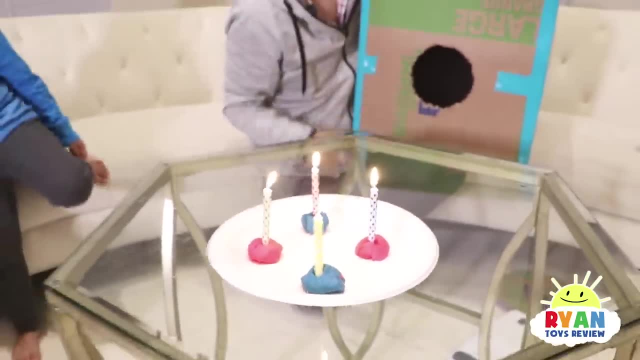 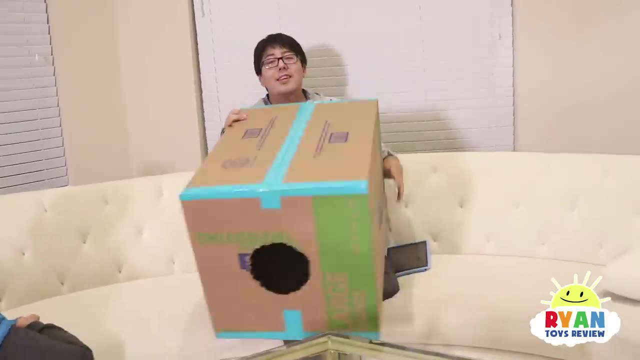 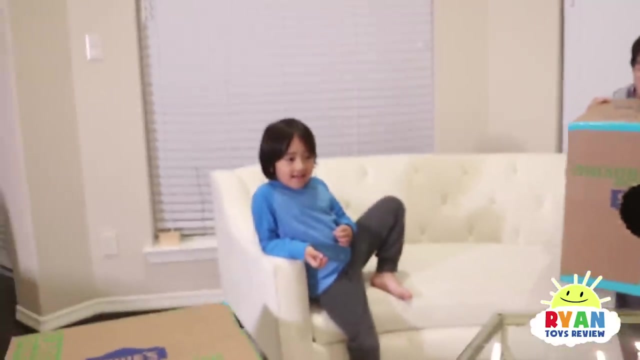 OK, guys, Before we start, do you think this air bazooka is strong enough to blow out the candles? What do you think, Ryan? Yes, Yes, OK. What do you guys think at home? Oh, the small one. 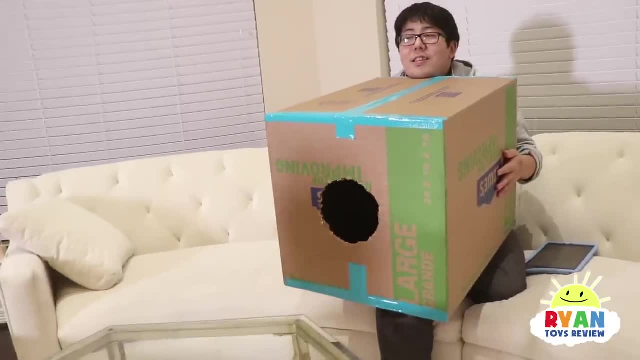 Yeah, So the small one, we already experiment that it's stronger, right? Yeah, All right, Let's see, Daddy, You guys ready? Yes, I'm ready, All right. Whoa, It blew out, except for one. 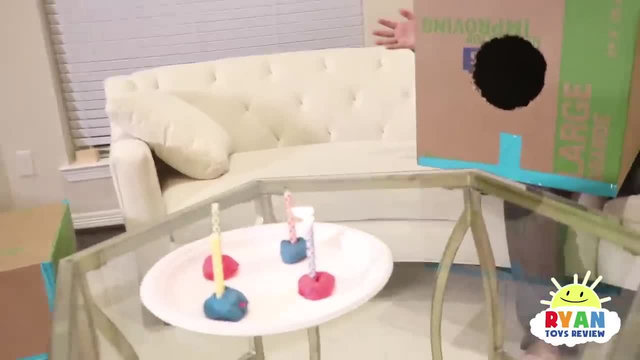 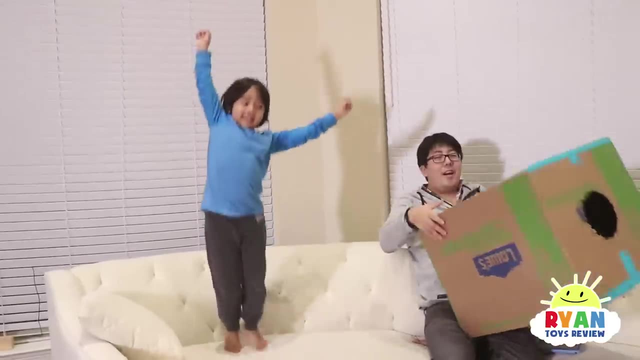 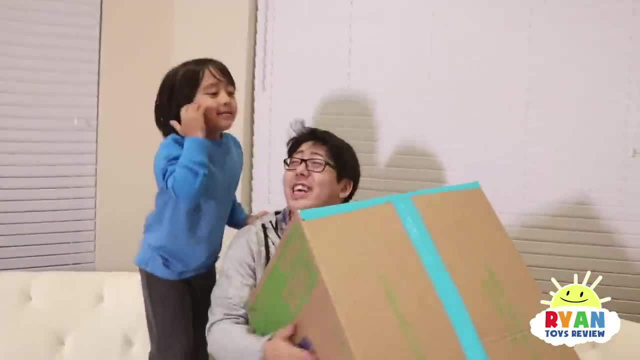 It feels good. It feels good The fan. it's not very hot. Yeah, if you're hot, you can use it as a fan. You can decorate your bazooka with faces. Whoa, That's funny. Look at him. he looks angry, grrrr. 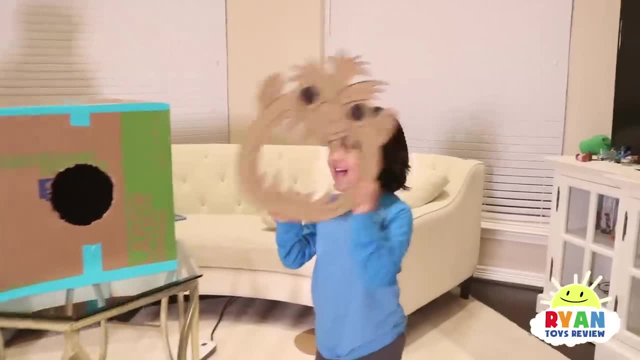 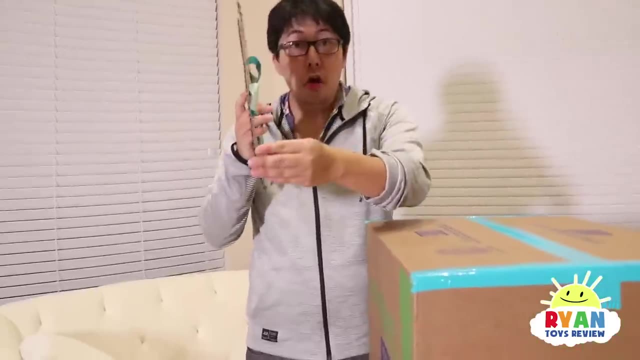 Put the duct tape on Boo Angry Daddy. Is it scary? He looks funny, scary, Funny, scary. Ryan has a fidget spinner for some reason. Yay, fidget spinner, Yay, Yay, Yay. 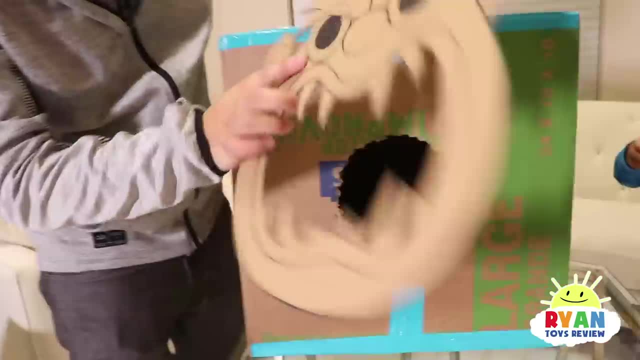 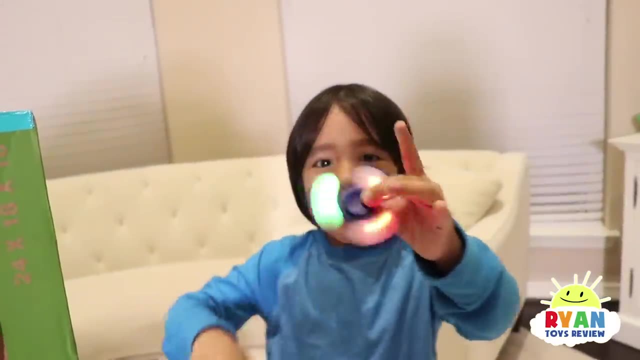 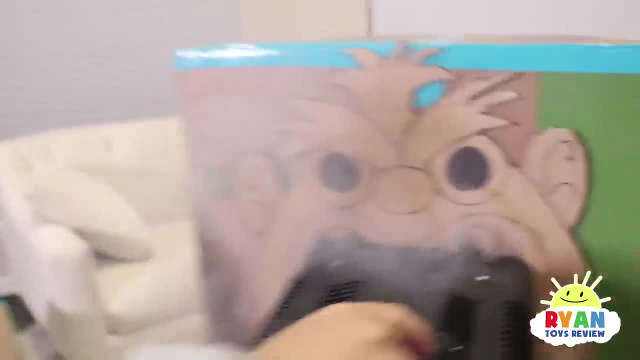 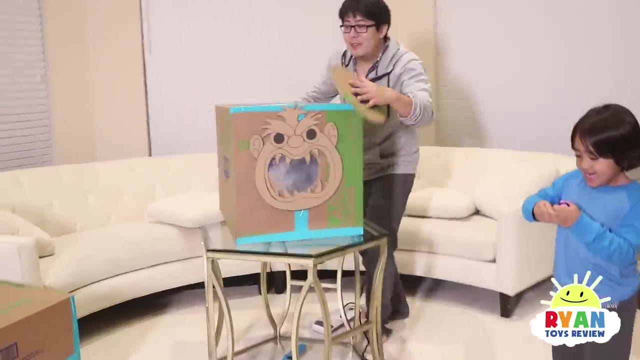 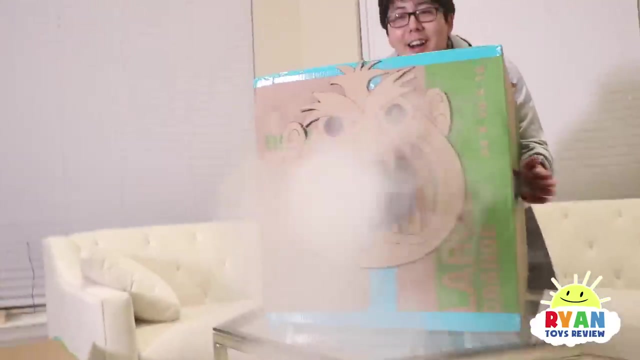 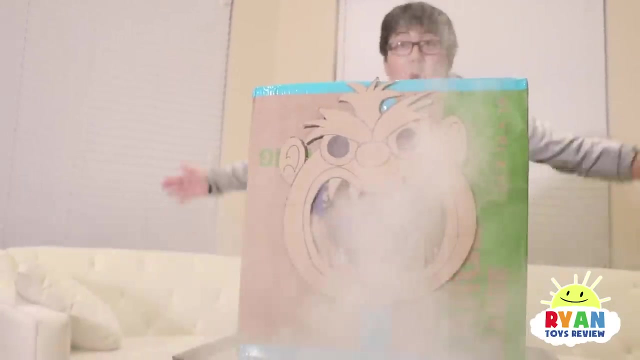 He's eating the smoke right now. He's eating pizza. He's eating pizza. Are you guys ready? Yes, That's a small one. Want him for the big one. Yeah, Whoa. Oh my, he just broke that thing. 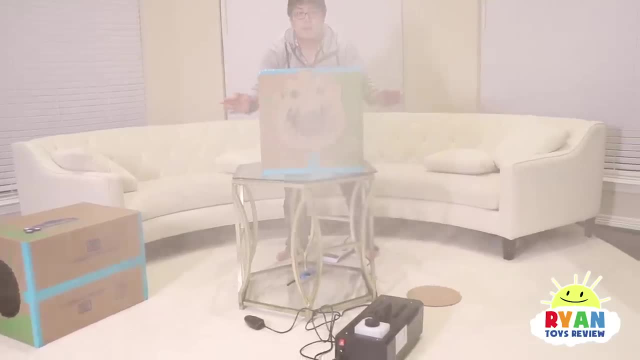 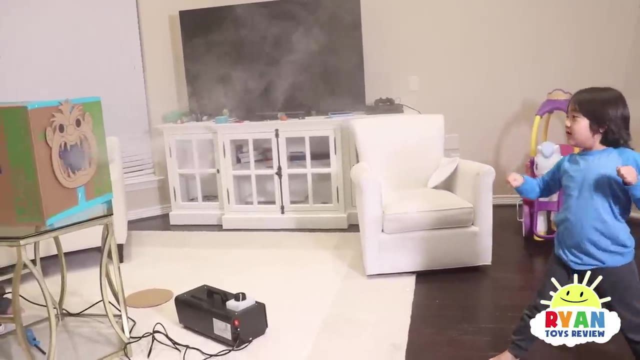 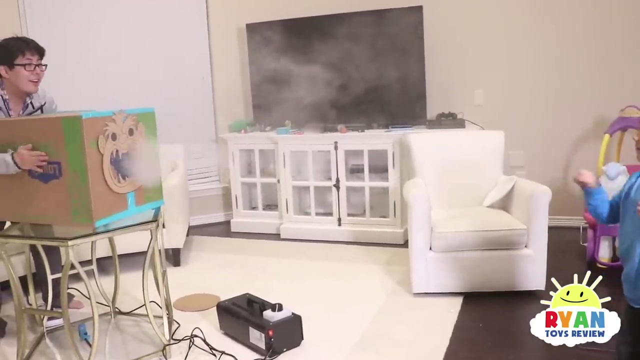 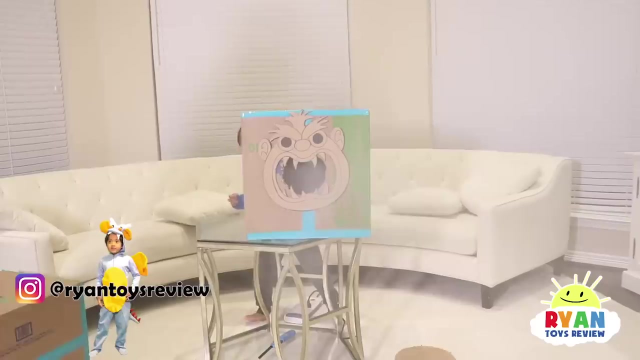 Are you cutting the hat? Whoa, So cool, He's punching the ring. I'll do a double ring, Okay, Whoa, yeah, you see the double ring. Wow, See, if you can do three, Am I doing it. 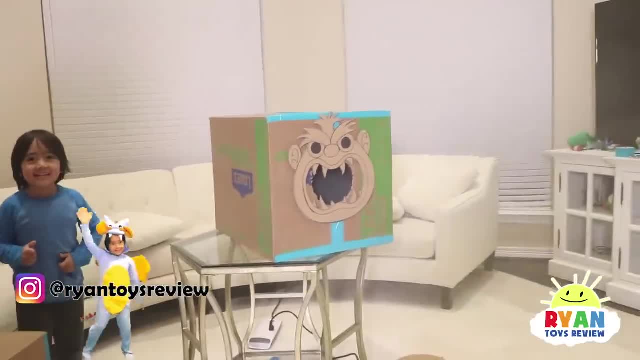 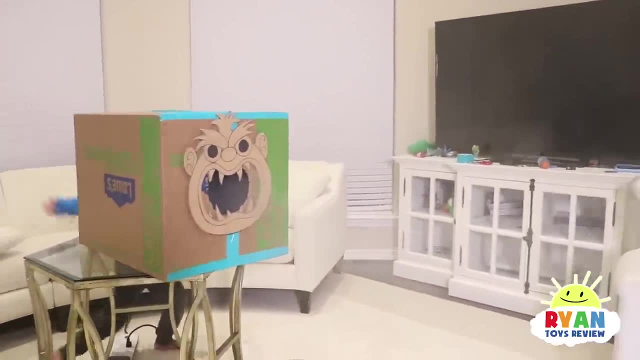 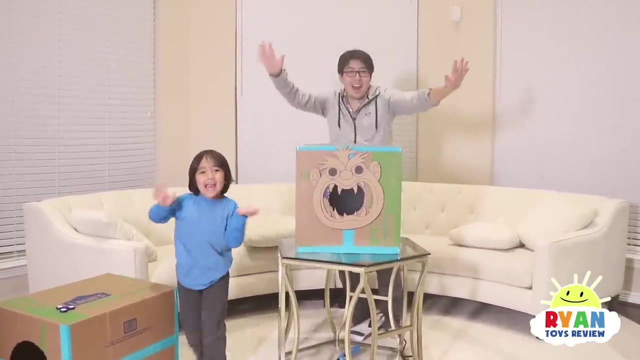 Yeah, Am I doing it? Yeah, Yours is coming out good. Yay, Thank you for watching our giant bazooka video. Bye, Bye everybody. If you guys do it at home, let us know, And if you do, do it, make even a smaller hole.